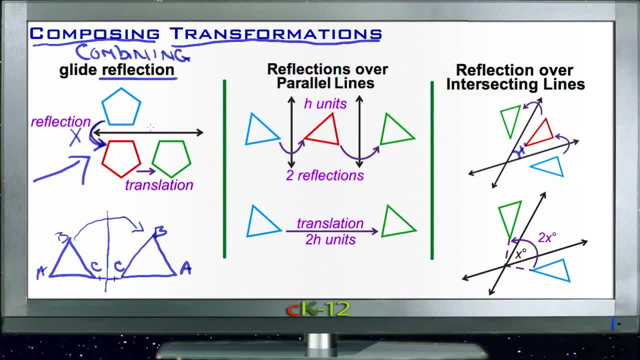 and we're reflecting it over the x axis, so reflecting it top to bottom, And then we're translating it or sliding it from right to left or from left to right- I mean to go from the red place to the green place. So this is a glide reflection, In other words. 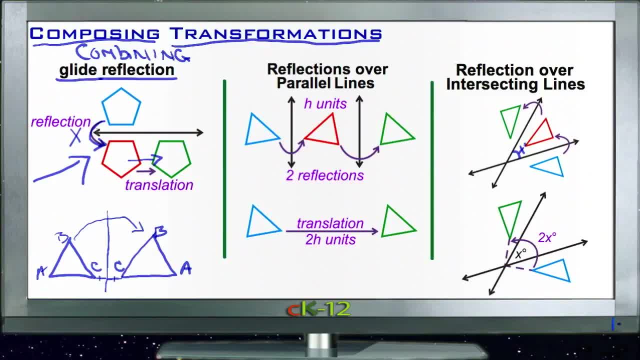 it's like a slide or a translation reflection. If we reflect over a parallel line in other over a parallel line. in other words, if we have, say, a blue figure here and we reflect it by h units, in this case we'll say: we'll pretend that this is a reflection of four units. 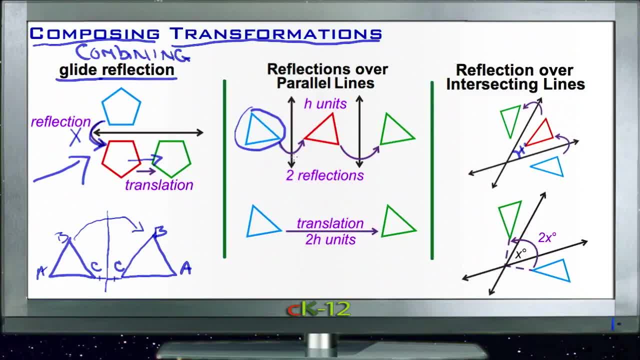 if i reflect it over this vertical line by four units, then that means that there's four units between this point here and this point here, and then another four units from this point here to this point here. so we have two parallel lines, and what we discovered is that if we were to 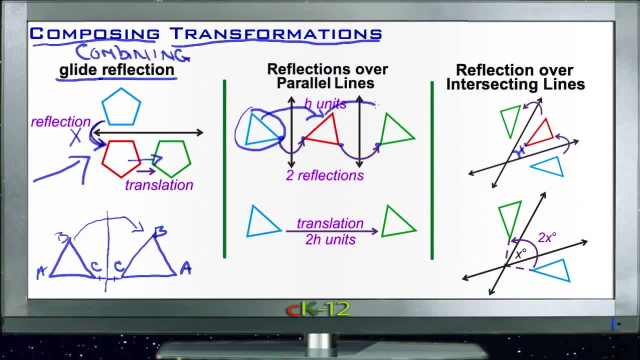 reflect it twice: first flip it over so it becomes red, and then flip it over again so it becomes green. it's going to be the same as if we'd just taken the original figure and slid it to the right, that same two distances that we originally flipped it. so if we go from blue to red by going four, 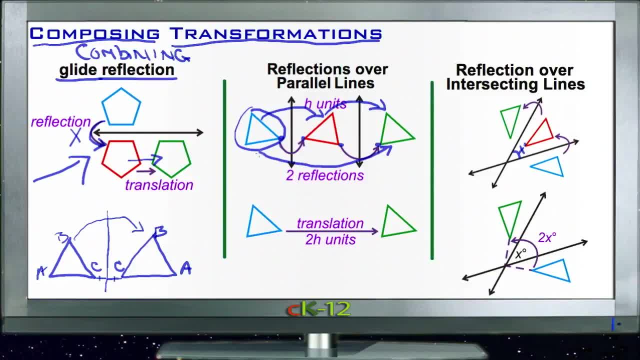 units and then from red to green by going four units. we could have just gone from blue to green by going eight units. so an h unit reflection over two parallel lines is the same as a 2h unit slide, because we flipped it twice. we flipped it and mirrored the image, and then we flipped it again and mirrored it again. 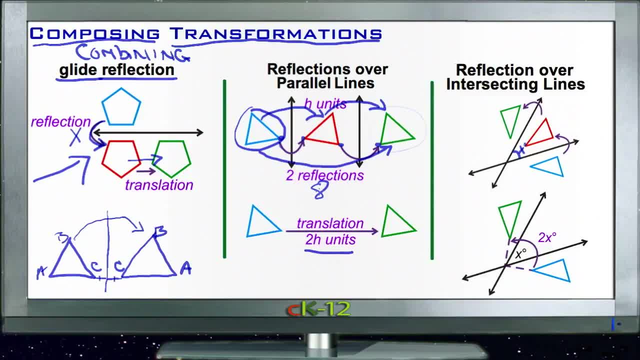 well, a mirror of a mirror is what we started with. i know that sounds confusing, but it's nice to know that you can simplify the process. instead of having to worry about actually flipping it over twice and seeing what happens, you can just slide the thing to the right and the same thing happens. 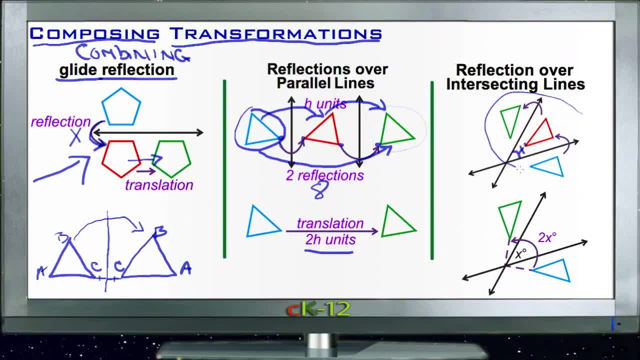 when you have intersecting lines. if up here on the top right, if i go from my blue figure to my red figure by reflecting over this angled line right here, and then i do it again and i go from the red figure to the green figure by reflecting over that angled line, again the same result. 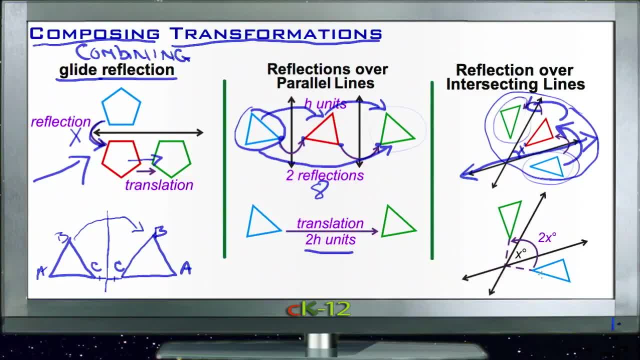 going from blue to green occurs if i were just to take my original blue figure and rotate it by twice, whatever that inside angle was, so if my original reflection from blue to red was a, you know, around an angle of 40 degrees, and then i'd do it again around an angle, that's another.